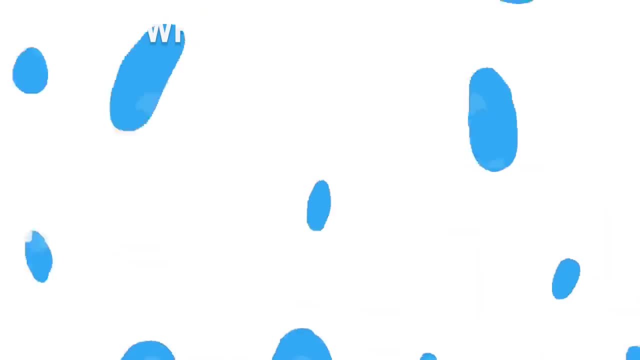 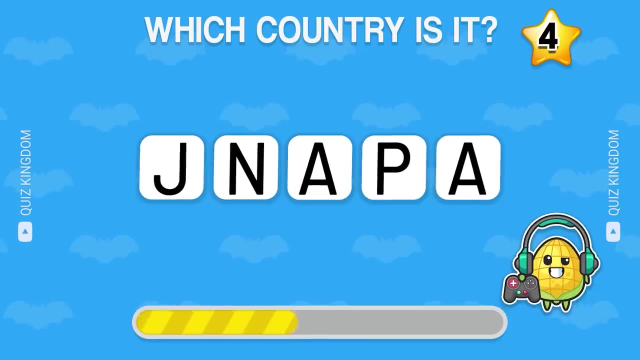 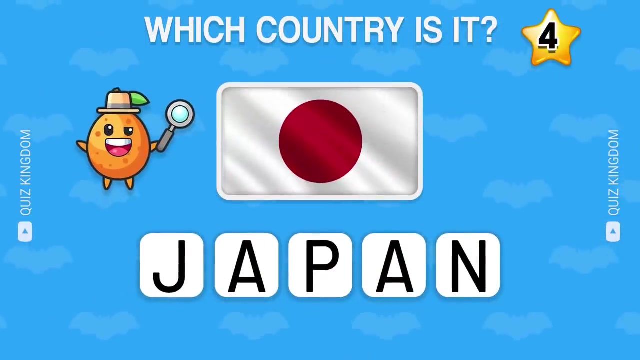 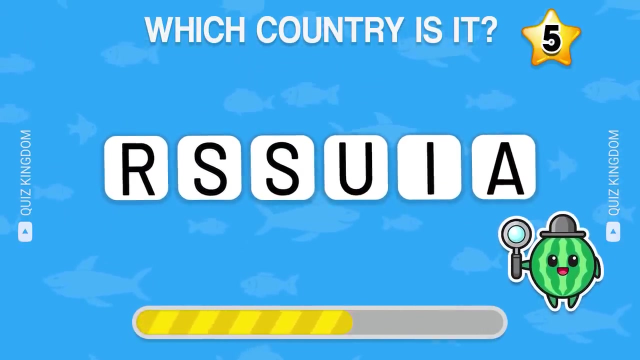 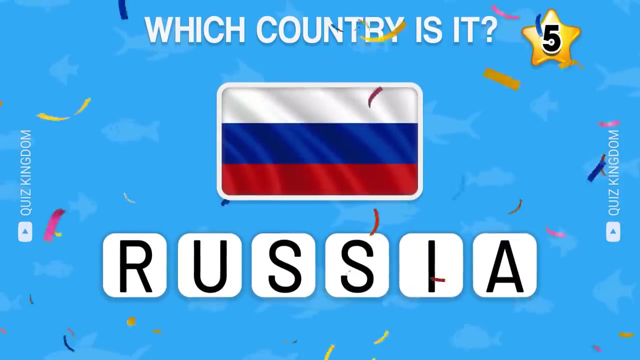 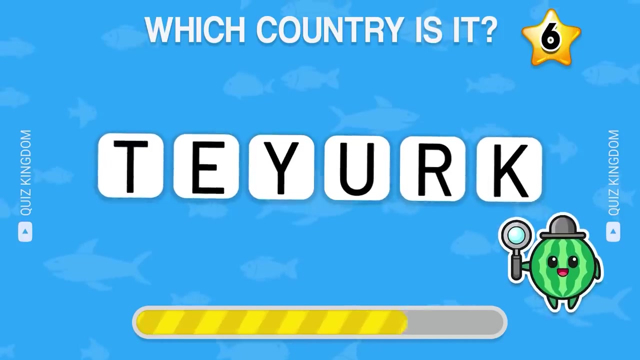 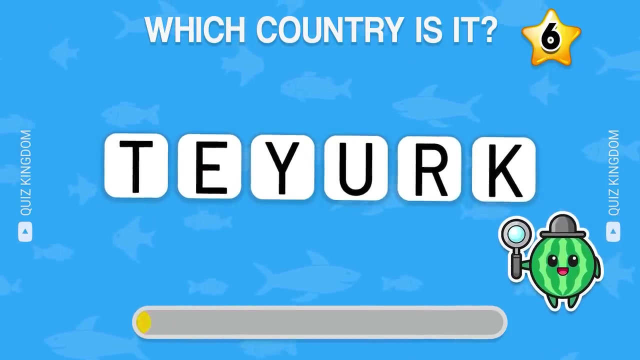 Wonderful. it's United Kingdom, Question 4.. Yes, it's Japan. It's the largest country in the world. Can you guess its name? You got it right: It's Russia. Can you guess the country? You're so good? it's Turkey. 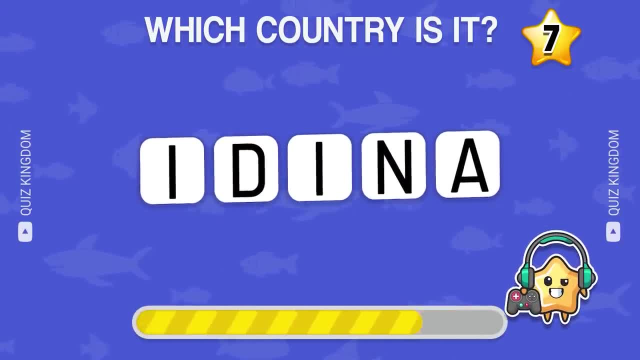 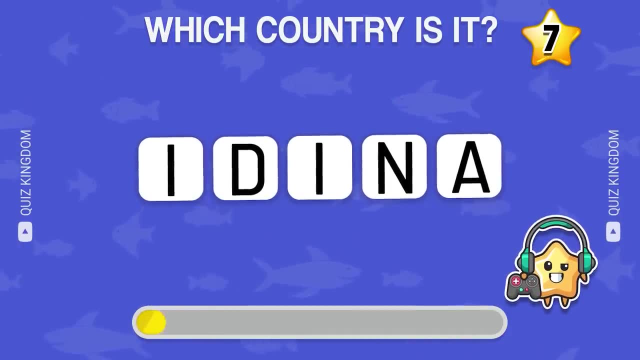 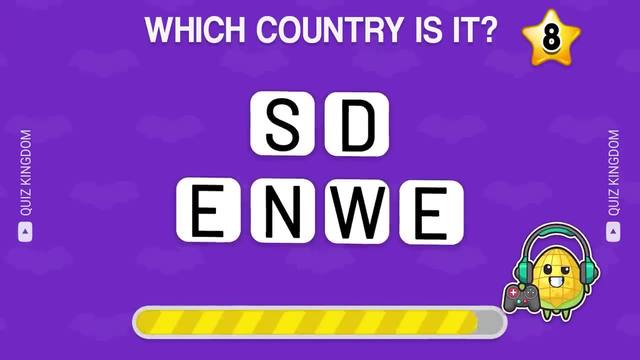 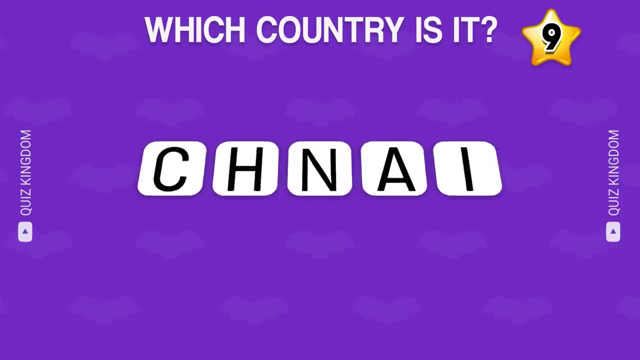 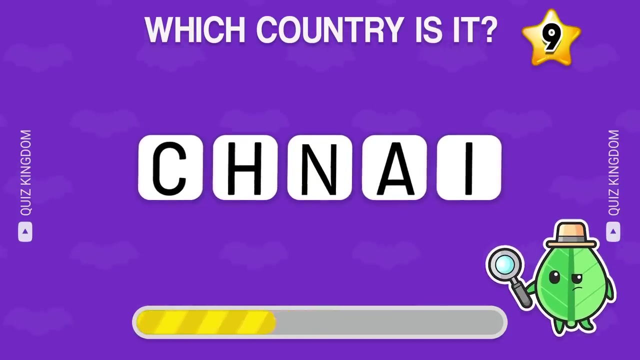 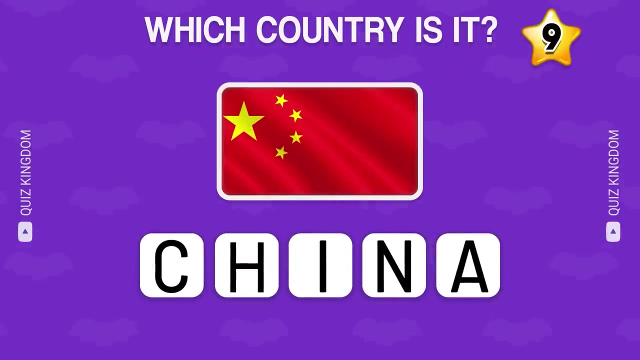 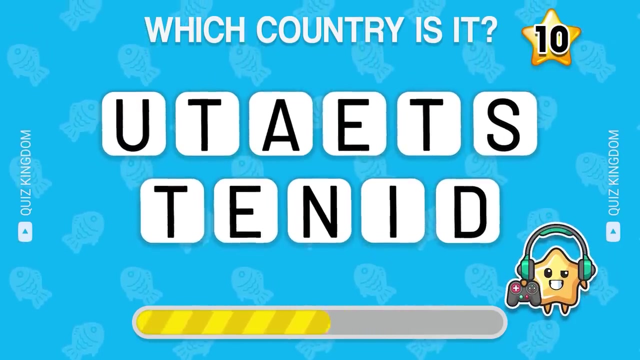 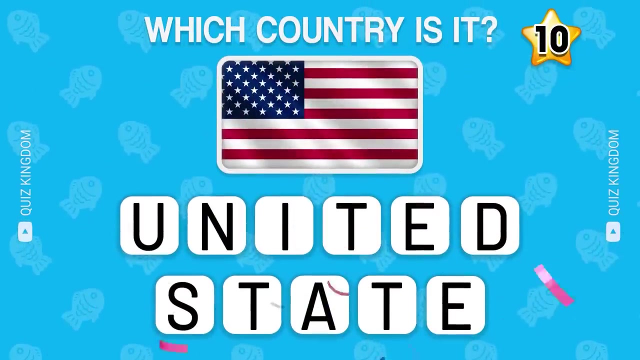 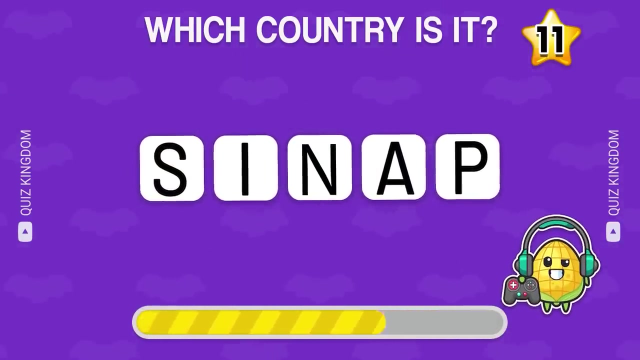 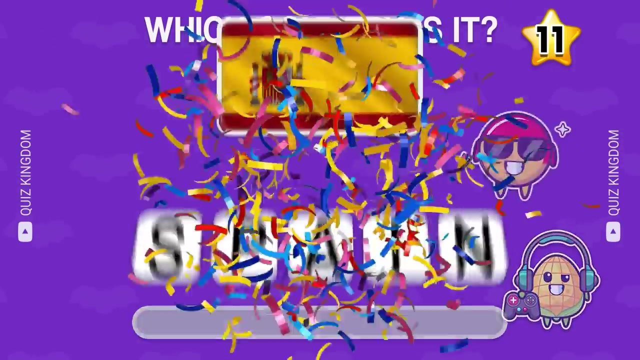 Question 7.. The country is India. Question 8.. Of course it's Sweden. Question 9. It's China. Do you know the country So great? it's United States. Can you see which country it is? The correct answer is Spain. 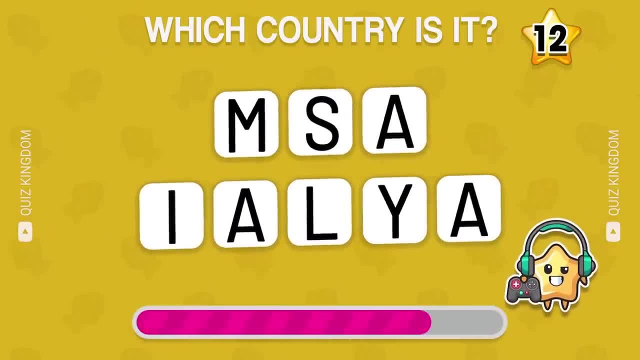 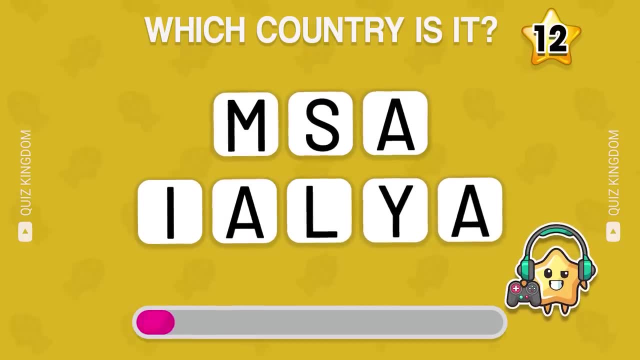 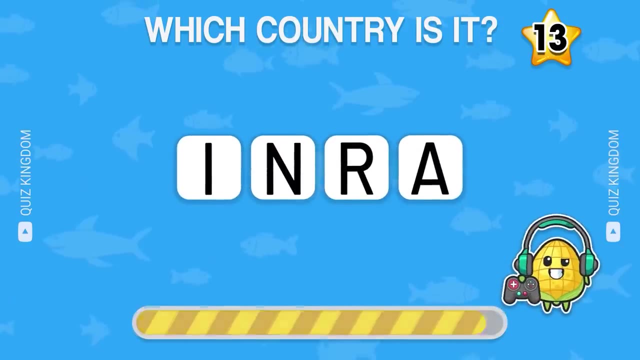 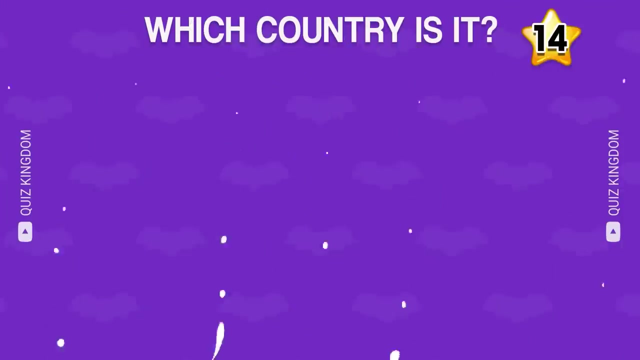 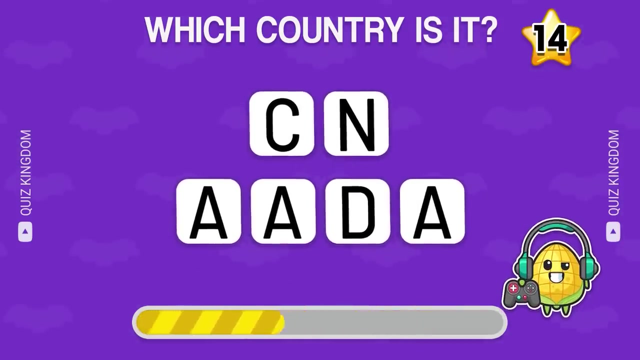 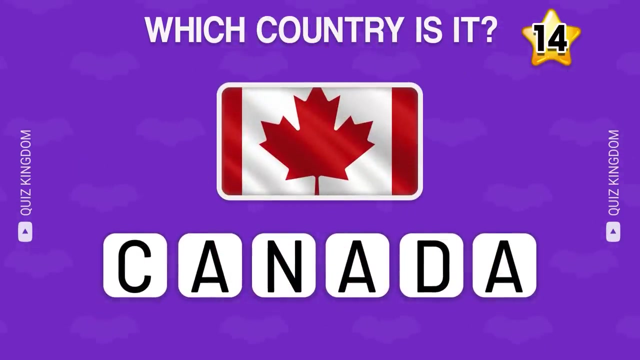 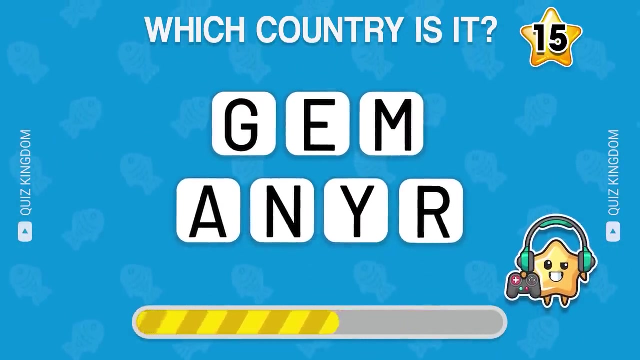 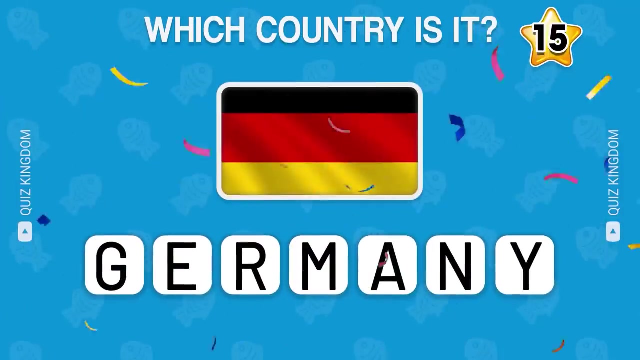 What about this one? It's Malaysia. Next up, the country is located in the Asia. Iran is the correct answer: Question 14.. The country is Canada. Can you guess the name of this country? You're so smart? it's Germany. 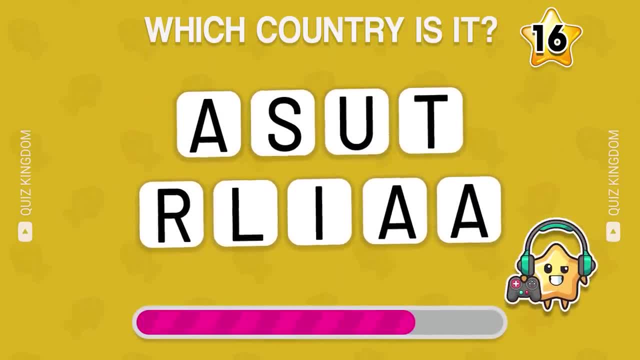 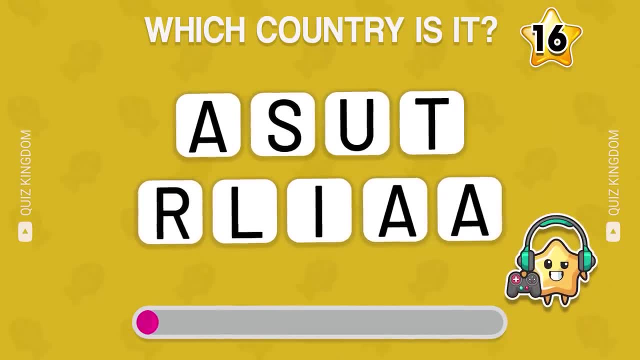 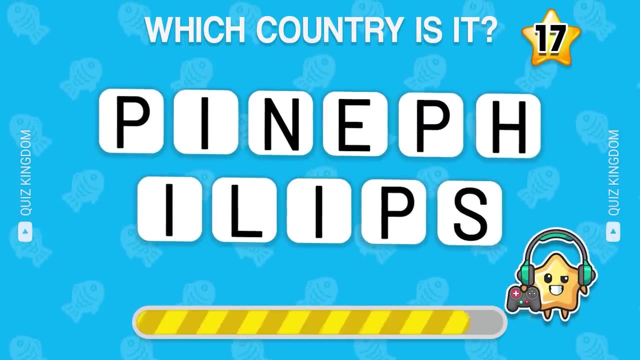 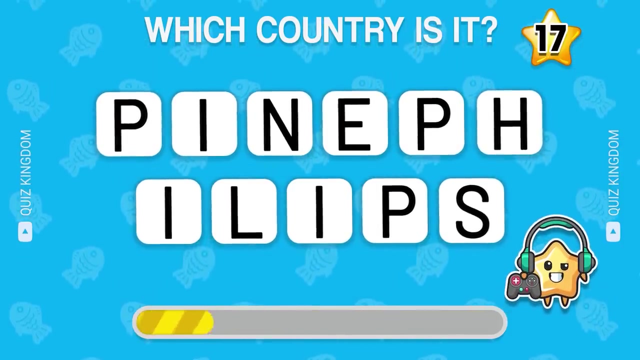 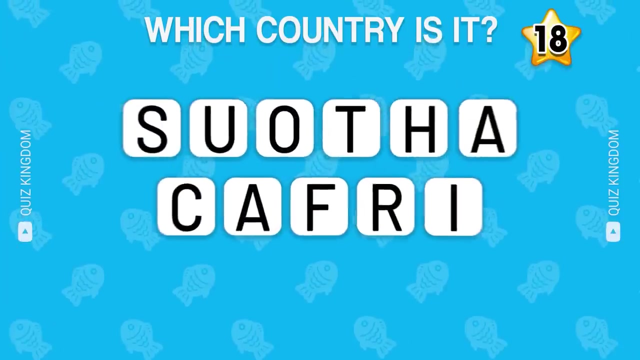 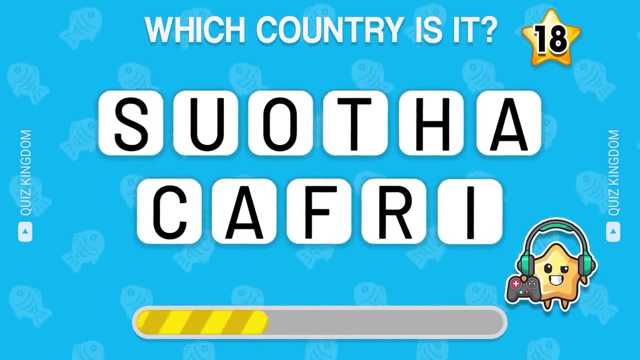 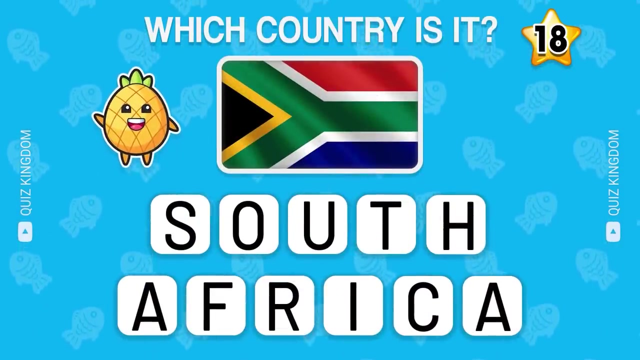 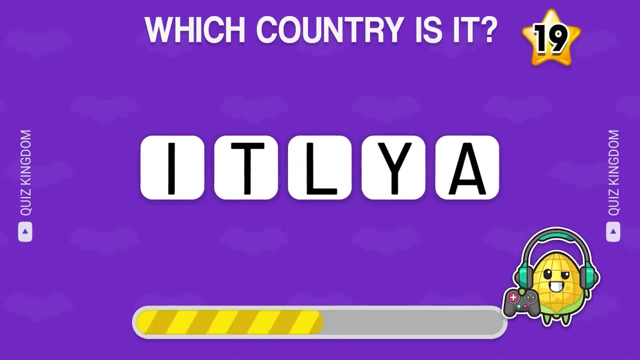 Next one, The country starts with the letter A. Perfectly, The answer is Australia, Question 17.. The country is Philippines. That's a long name. Can you guess? It's South Africa. What about this country? It's Italy. 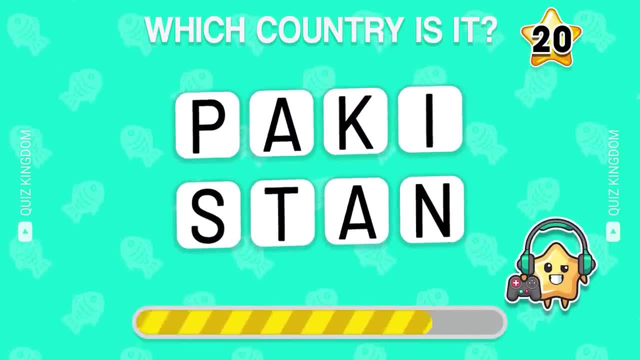 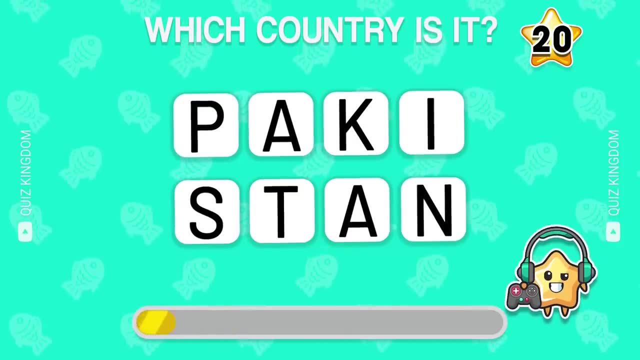 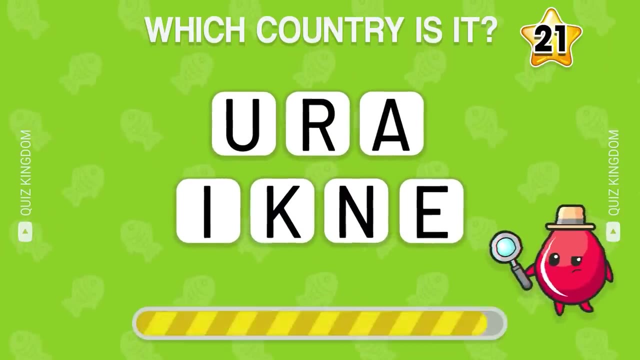 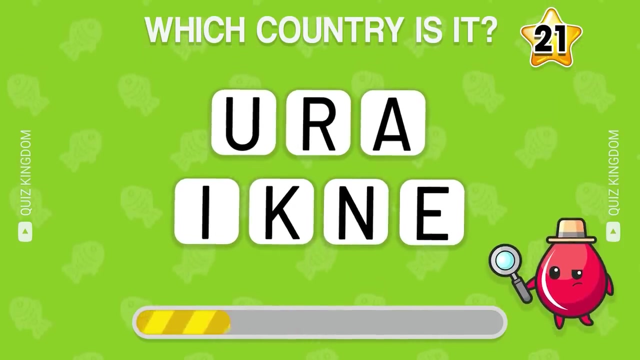 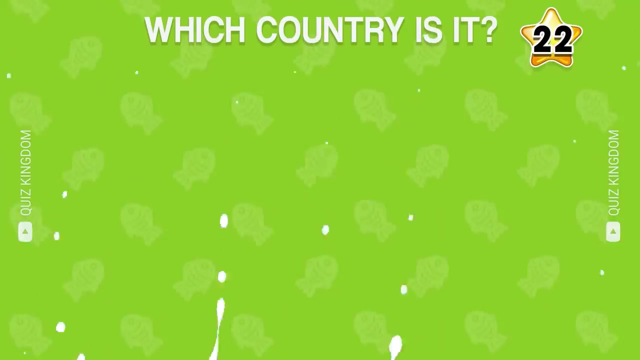 Question 20.. Of course, the correct answer is Pakistan. Next country: The country starts with the letter A and it starts with the letter B and it starts with the letter A. Great, it's Ukraine. Which country is this? 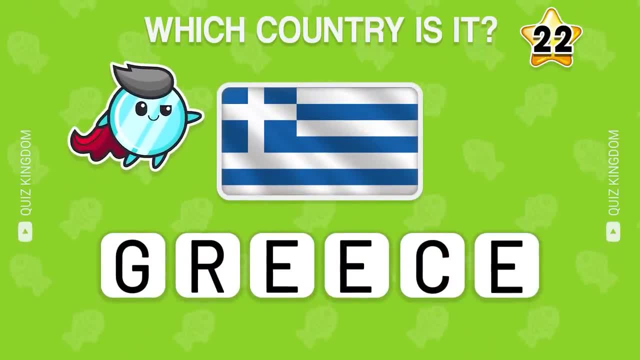 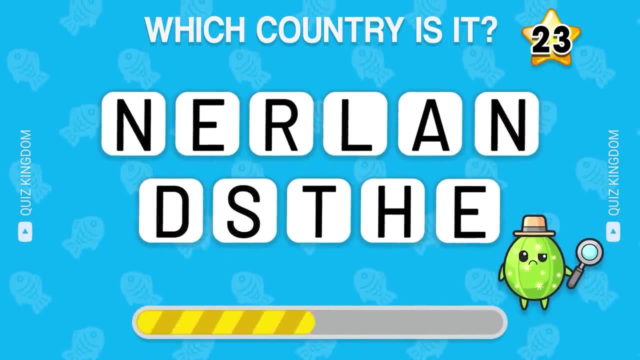 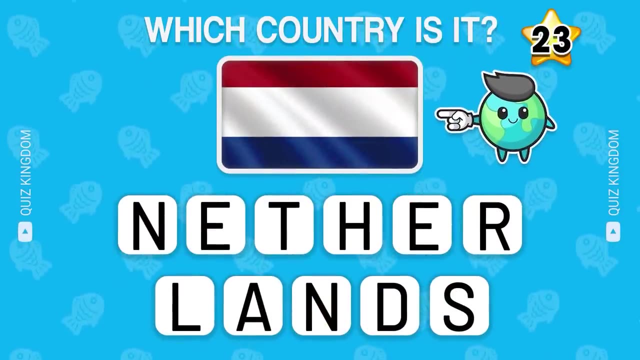 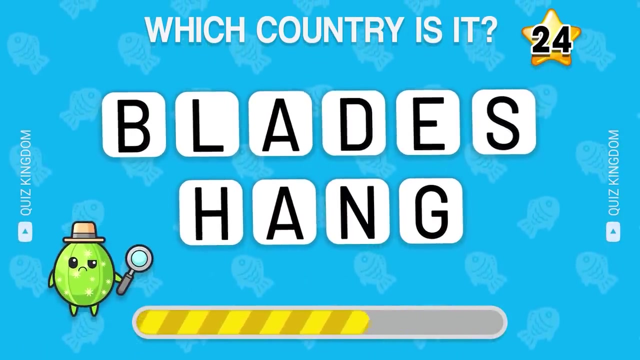 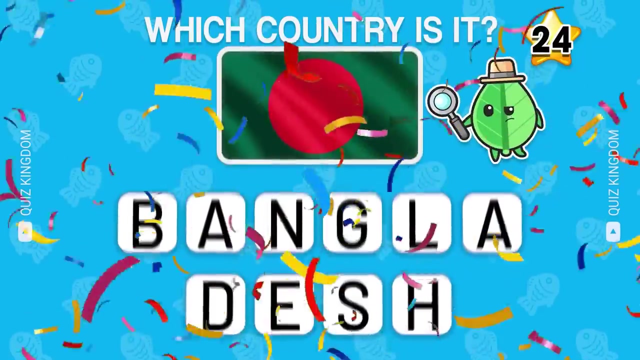 Time's up. It's Greece, Question 23.. The country starts with the letter B and it starts with the letter B and it starts with the letter A. Correct, It's Netherlands, Question 24.. That's good, It's Bangladesh. 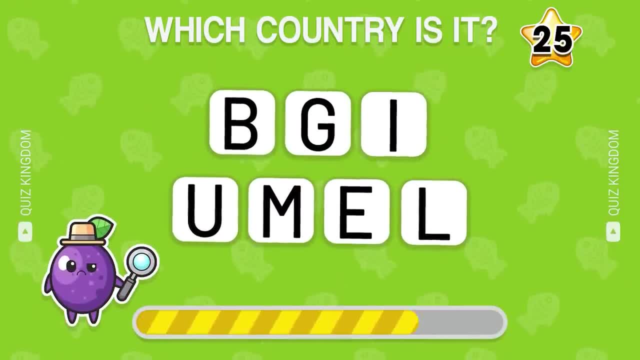 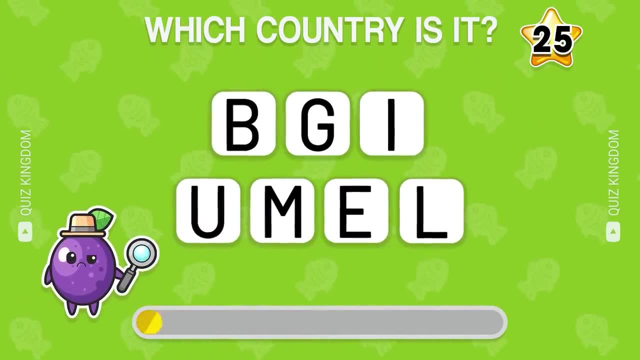 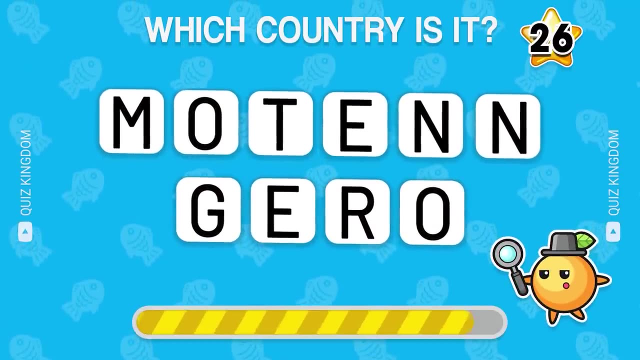 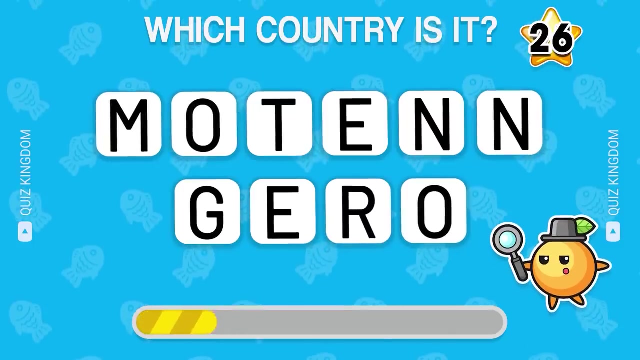 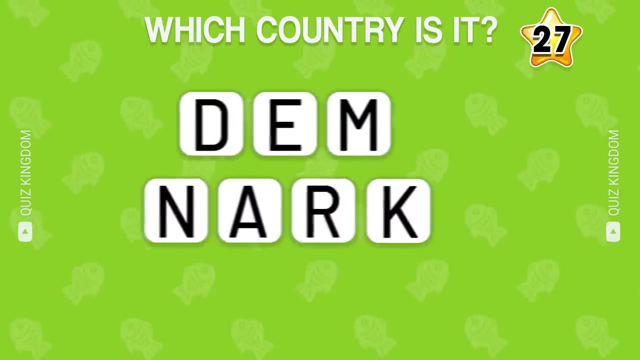 Can you guess the country? It starts with the letter B. It starts with the letter B. It starts with the letter B. Excellent, The country is Belgium. What about this one Great answer: It's Montenegro, Question 27.. 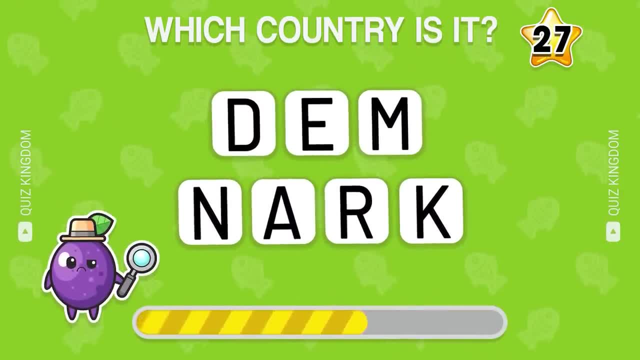 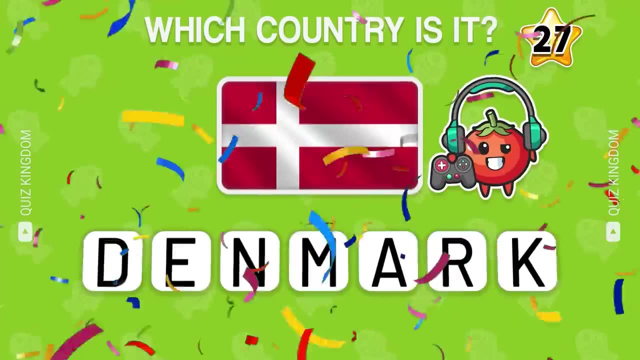 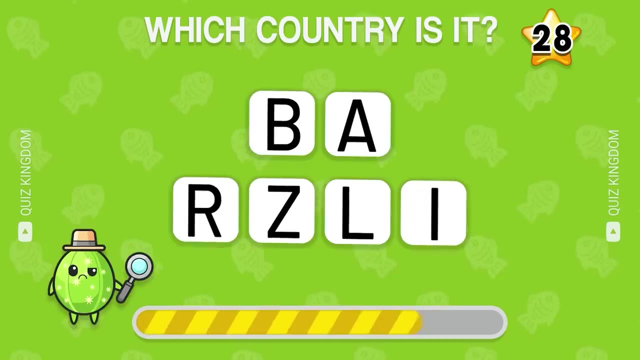 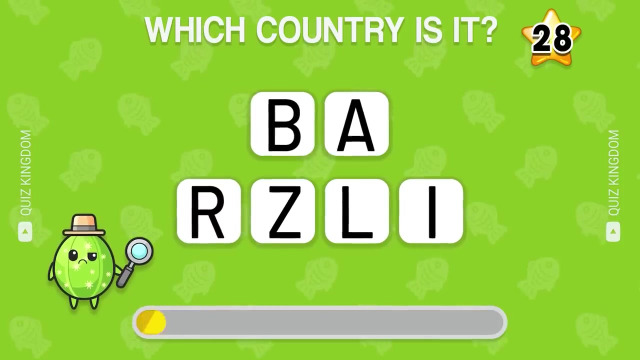 The country starts with the letter B, and it starts with the letter B and it starts with the letter A. So good, The correct answer is Denmark. It's the largest country in South America and in Latin America. That's right. It's Brazil. 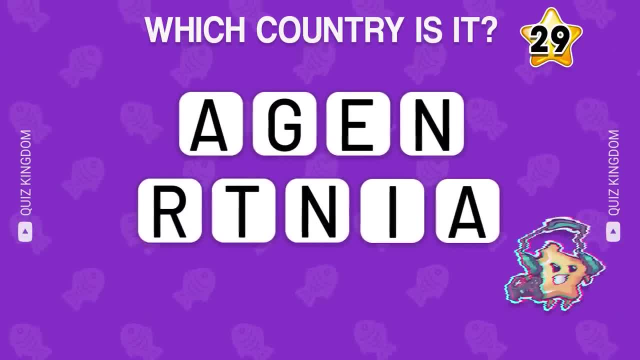 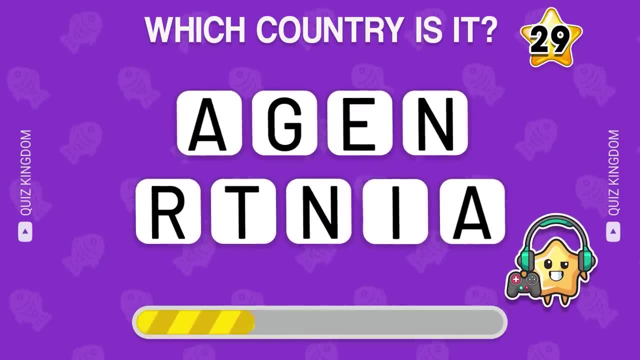 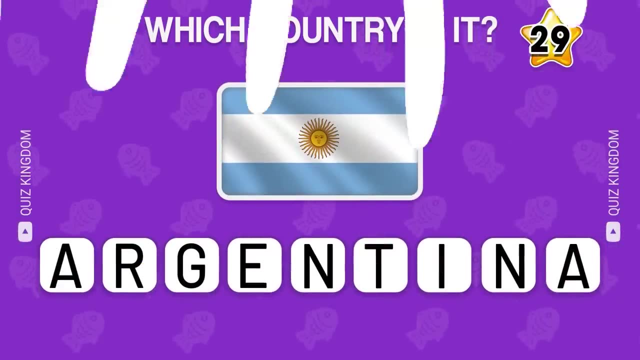 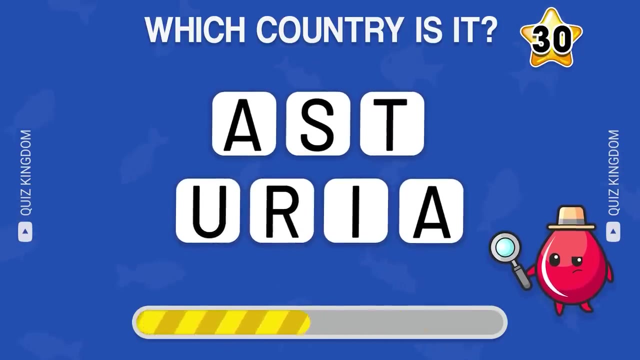 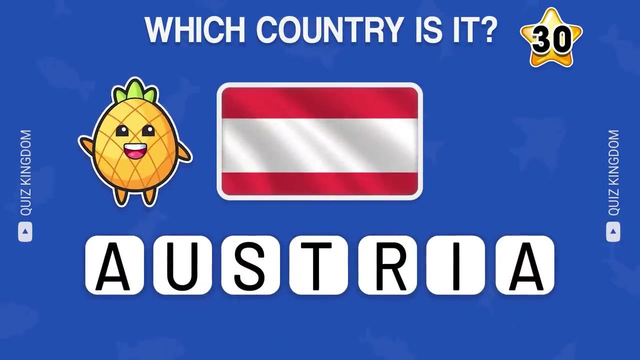 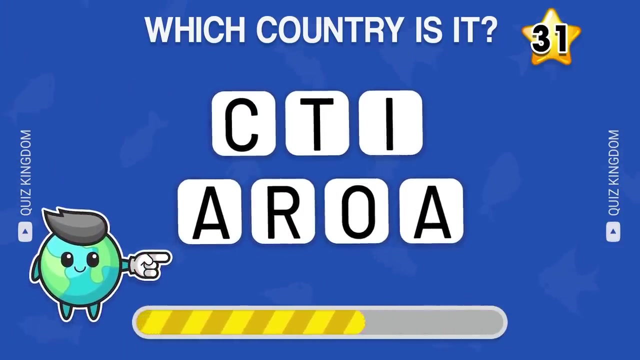 It's Brazil, Question 28.. This country is known as the birthplace of many football legends. So good, It's Argentina. Next up, which country is this? Awesome, It's Austria. Good answer: Question 31.. It's begginer that probably comes up. 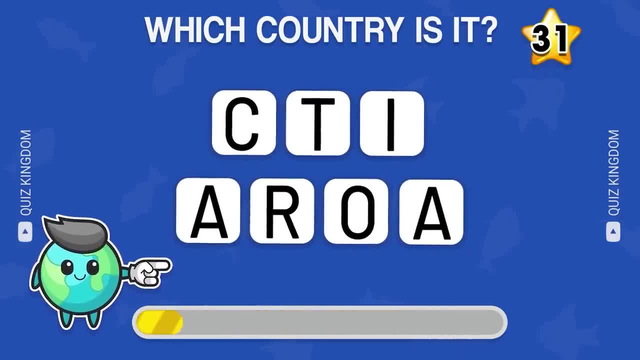 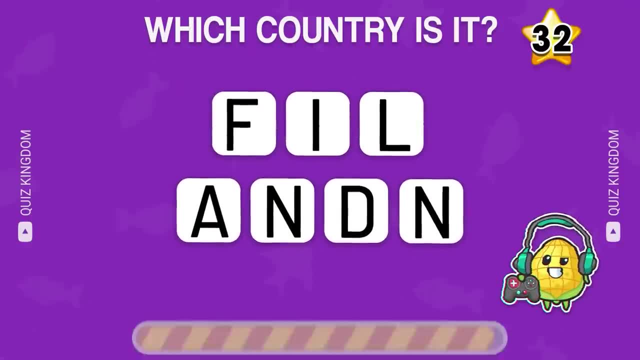 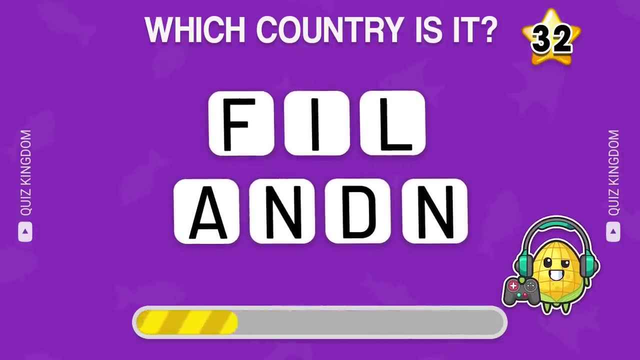 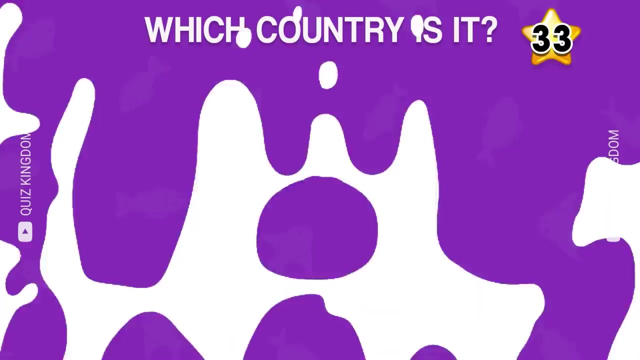 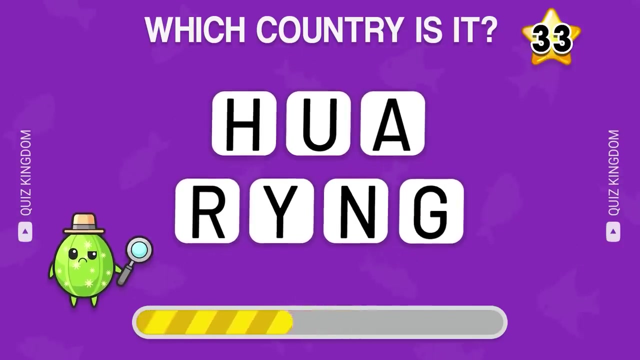 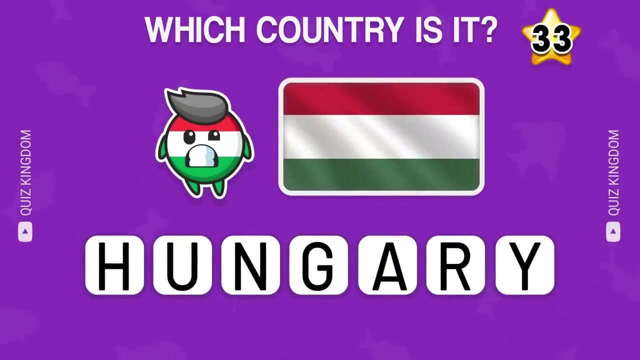 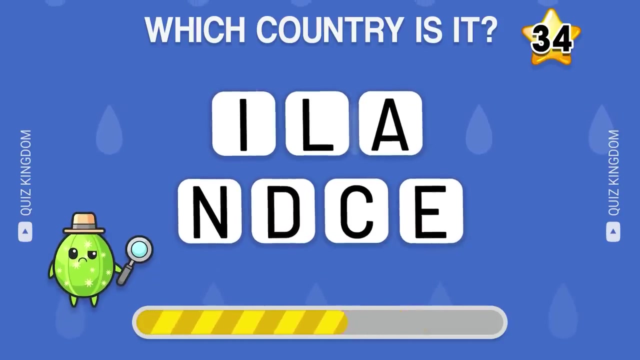 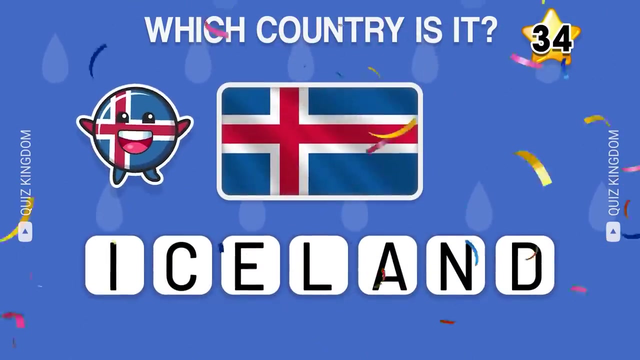 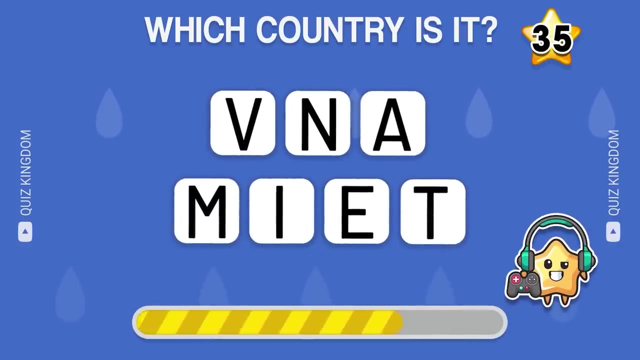 Great answer: It's Hungary. What about this country? It's Croatia. Correct, It's Croatia. Do you know this country? Time's up, It's Hungary, Question 34.. It's Iceland. Can you guess the country? Wonderful? It's Vietnam.